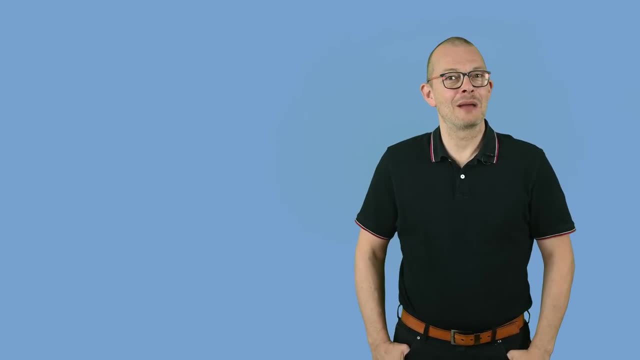 Great learning experience. As I wanted to make a video on IPv6 for a long time already, I thought – how would I transmit that learning experience to a similar audience? So here is the idea of this video – you forget everything you know about IPv4.. 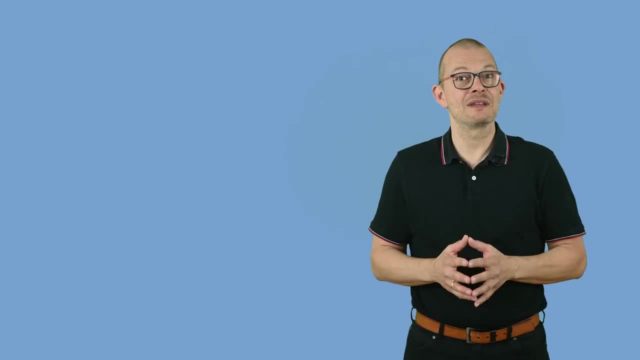 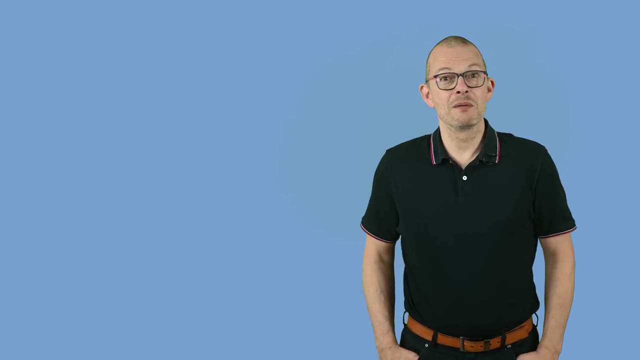 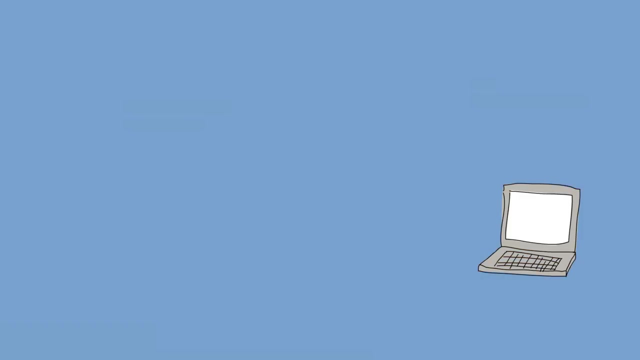 And we will design a new protocol – IPv6 – from scratch. Together. We will do as if there was no protocol at all and as if we would need to design it From nothing. Shall we do that? Let's go. We have two nodes here: PC, phone, tablet, anything. How can we connect them? How can 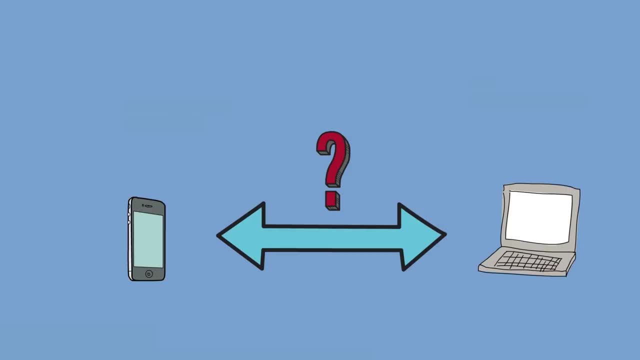 we build a network and have them talk to each other I'd say – each of these needs an IPv6 address, Like homes in the real world have addresses, As those devices are computers and as computers know zeros and ones – also known as bits – let's just think quickly how. 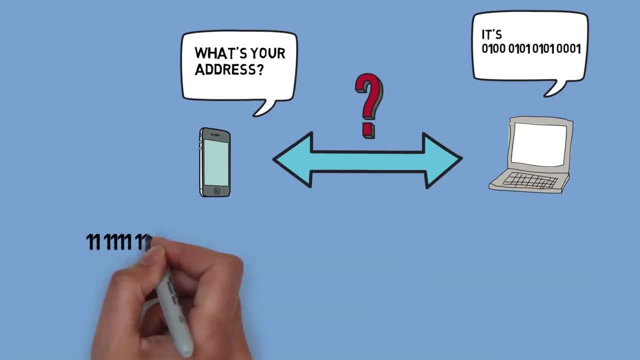 many bits we would want to give away for an IPv6 address. If we used 10, then we would have 2 to the power of 10 different addresses available. That's 1024 IPv6 addresses, Not enough for this world If. 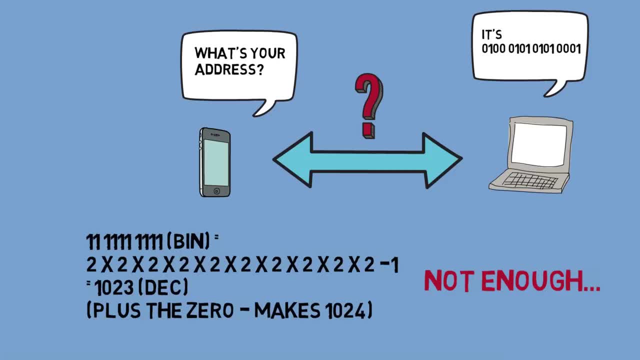 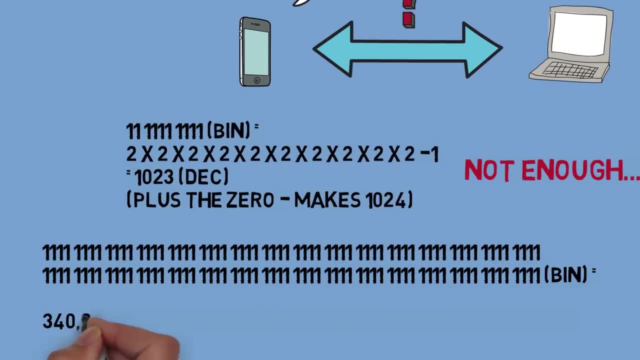 we used 128 bits, or in other words 16 bytes – that's really not much memory these days – then our IPv6 could use 2 to the power of 128, which equals, ehhh, gazillions of addresses. That should do. Let's rather go large – our IPv6 addresses shall hence be 128 bits large – that's. 16 bytes. This way we can nicely group them in, lets say, 8 groups of 2 bytes. If we write the groups in hex numbers – that's 16 bytes- then we should be able to link everything together in our IPv6 address. 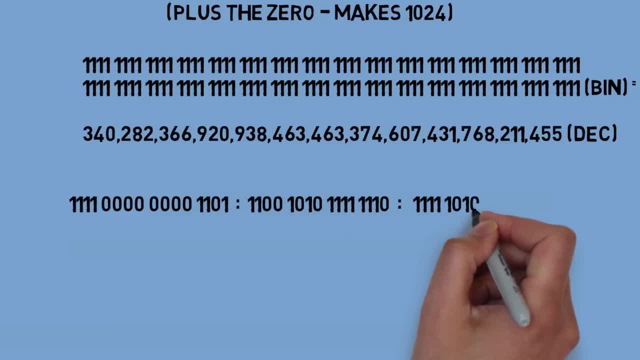 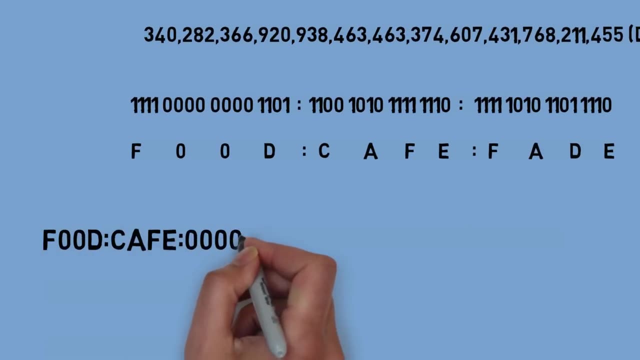 hex numbers, then we would have 8 blocks of 4 hex digits. This way, people could even build short words with the blocks, such as food or café or fade or whatever. In order to separate the blocks, let's arbitrarily choose the colon character. So a valid address. 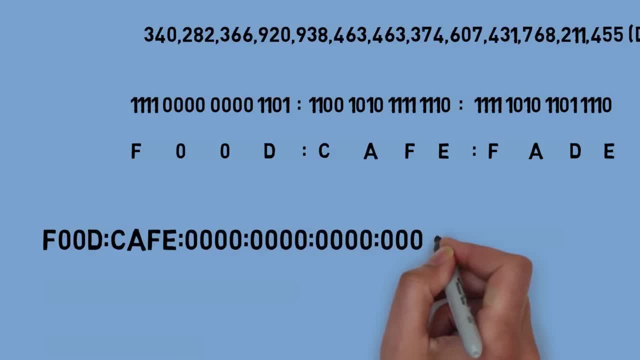 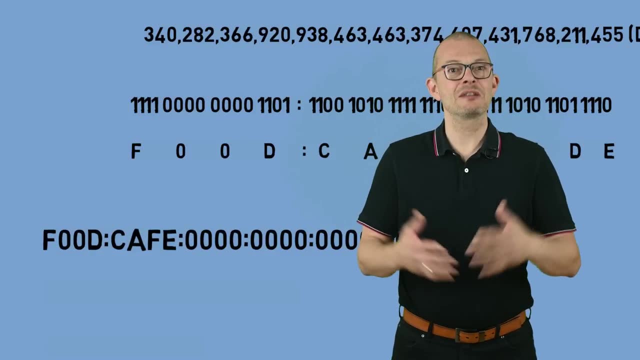 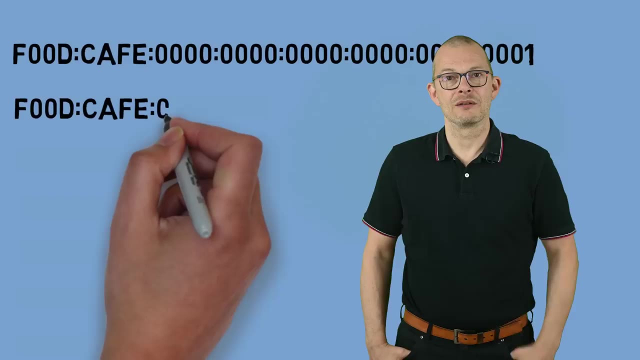 would be food colon, café colon, many zeros with colons and then colon 0001.. Just one thing is annoying here: This IPv6 address is long, Let's shorten it. Let's remove leading zeros in each block. In this case, that would be food colon, café colon 0001.. 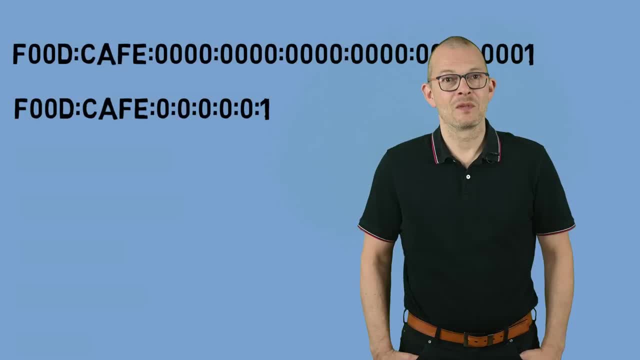 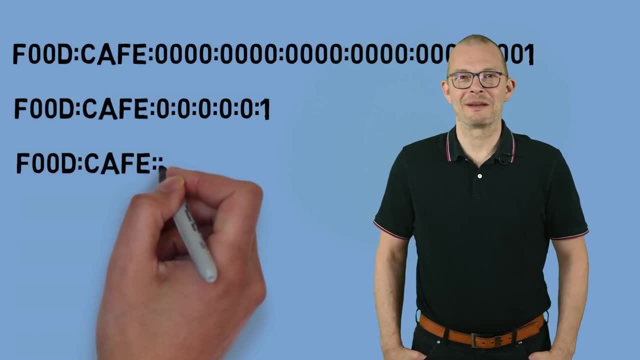 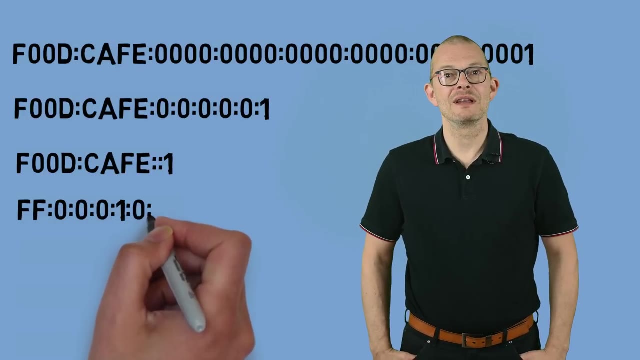 You know what? Let's not write the zeros at all, Let's just write a double colon instead. So food colon, café colon, colon 1.. Looks much better. Just, we can only do this once in order to avoid ambiguity. ff, colon, the many zeros, colon 1, colon 00, colon 1 could hence be written like this: … or 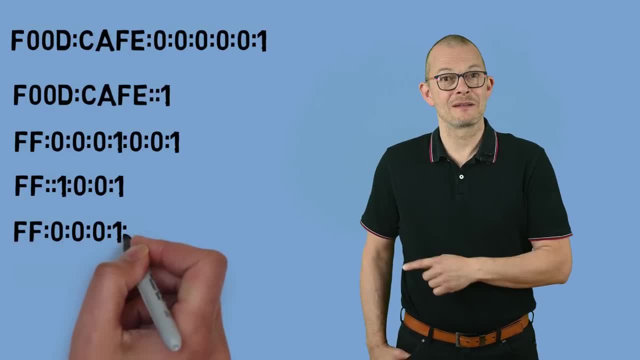 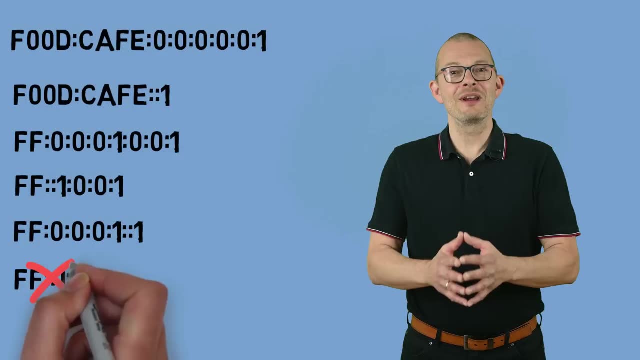 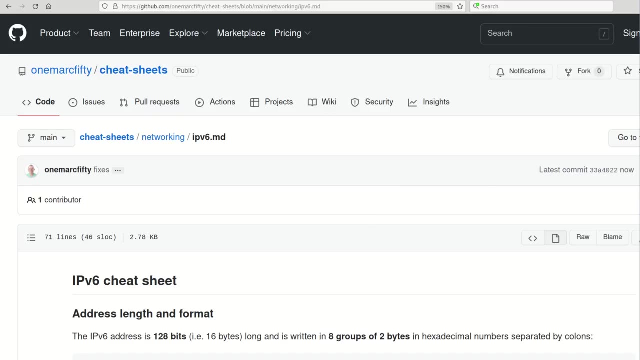 like this … but not like this … because we would not know how many zeros to put into which block. Let's stop here and write down our findings on the 1mk50 IPv6 cheat sheet. We can use this later to look things up. IPv6 address. 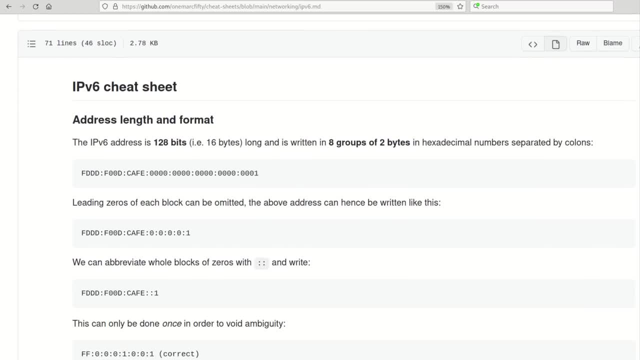 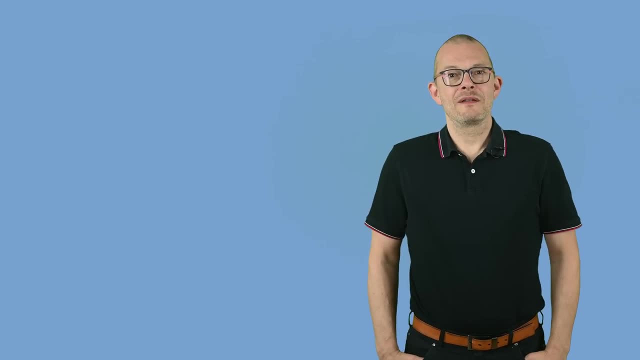 length, How to shorten IPv6 addresses, How to abbreviate zeros in IPv6.. Here we go. So now we have these two or three IPv6 nodes that can talk to each other. Just, we might need one more thing. We need to specify how they talk to each other. If we were sending 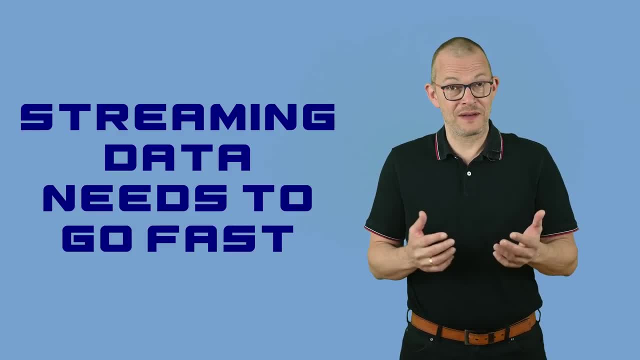 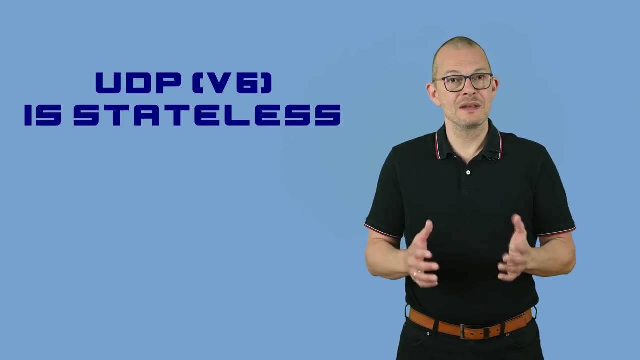 voice or video data, then we would go as fast as possible. In turn, it doesn't really matter if we lose a packet or two. Let's therefore create an IPv6 protocol and call it the User Datagram Protocol, or short UDPv6.. This IPv6 protocol will be stateless – that means we just fire and forget packets. 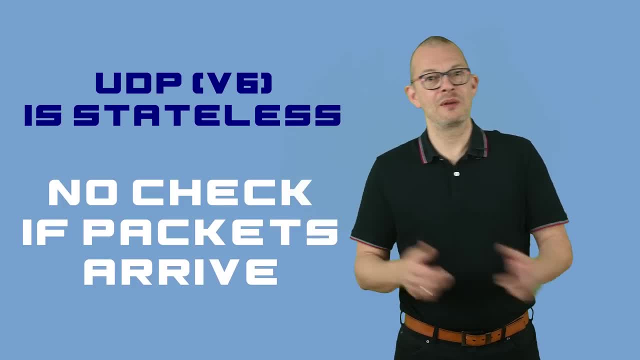 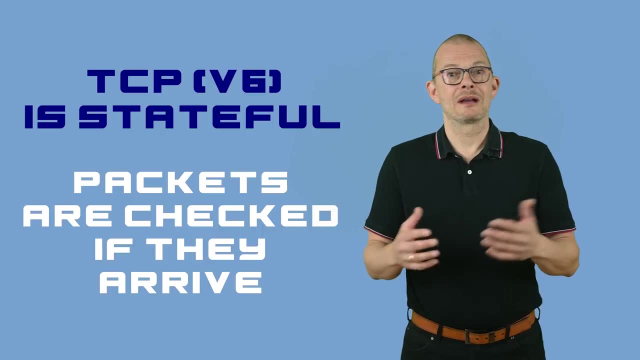 and do not check if they have arrived, We just throw the IPv6 packets over the fence. On the other hand, if we need to make sure that all IPv6 packets have arrived, kind of like with the registered letter at the mail where the recipient signs that it has arrived- 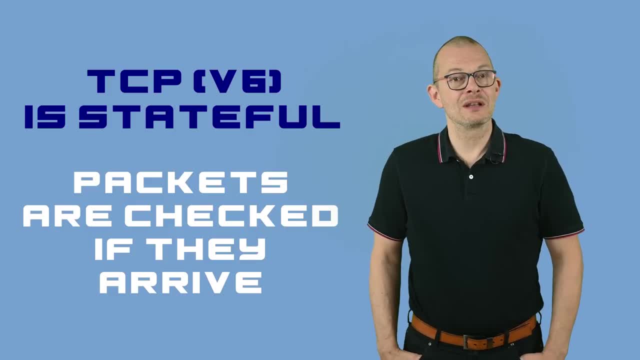 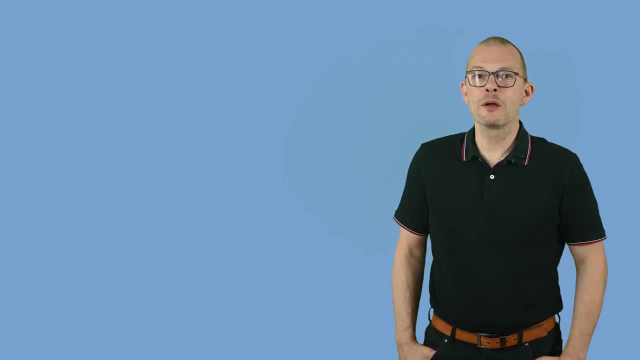 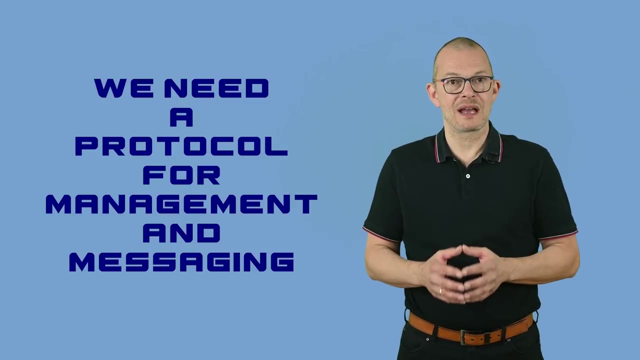 we use another IPv6 protocol. Let's call it Transmission Control Protocol or TCPv6. But we have a third use case, actually a bunch of use cases. How are we going to tell those nodes which IPv6 address they will be having, for example? How are we going to announce to them? 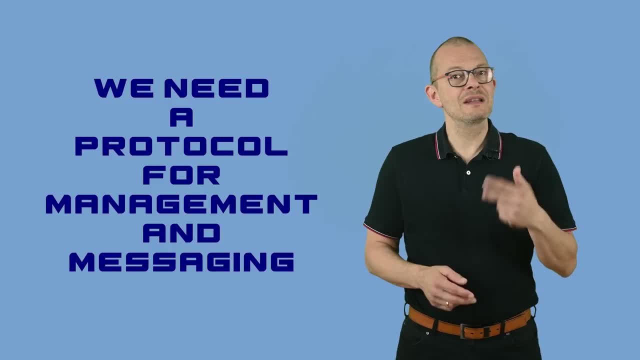 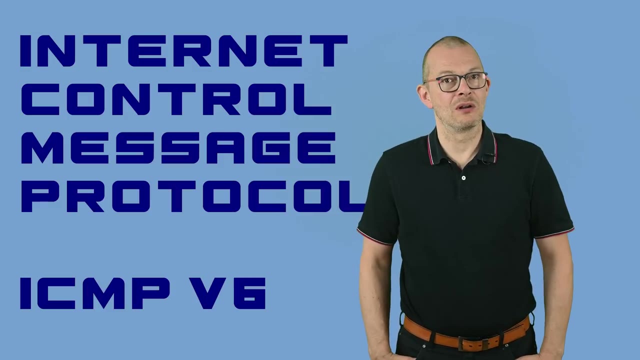 that there is an IPv6 router which they can use. Let's define a third IPv6 protocol which we will basically use to manage, or rather control, everything in our IPv6 world. Let's call this protocol Internet Control Message Protocol, or short ICMPv6.. Let's assign numbers to those. 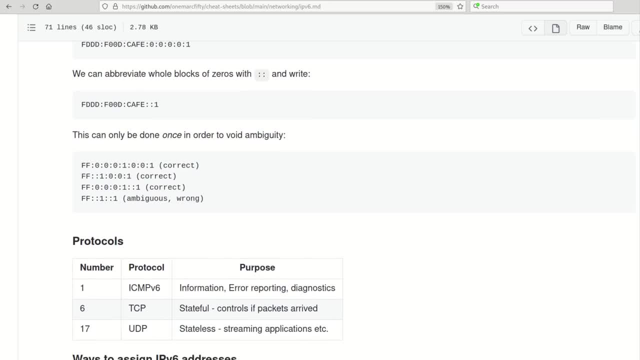 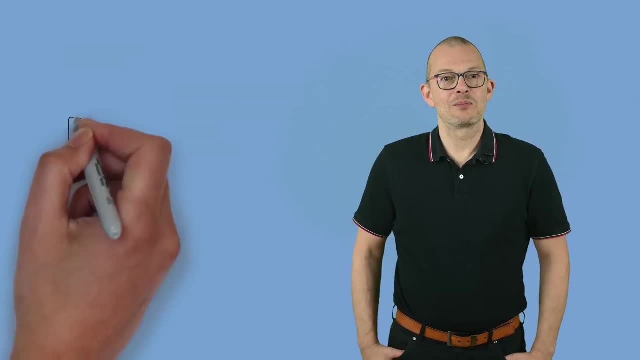 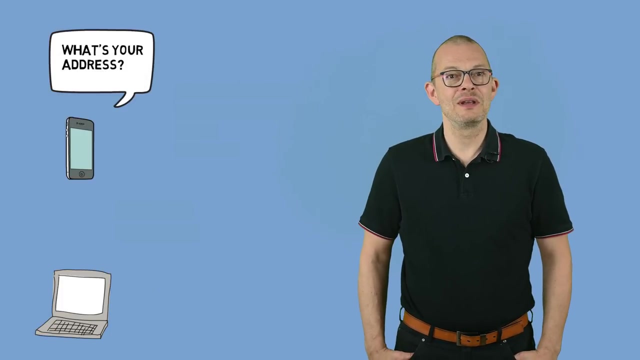 IPv6 protocols and quickly write them down on the IPv6 cheat sheet. We have one last problem to solve: How are we kicking everything away? We have one last problem to solve: How are we kicking everything away? That means, how do we start ICMPv6 communication with the nodes if they don't have an address yet? 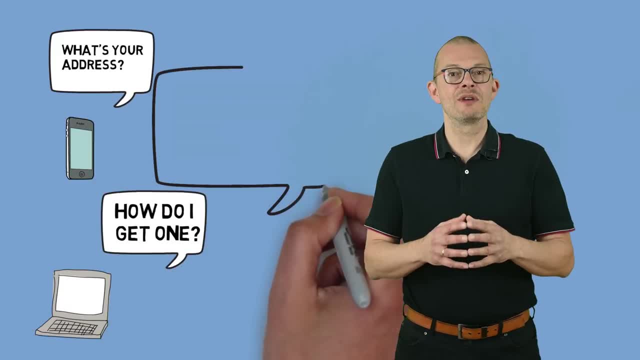 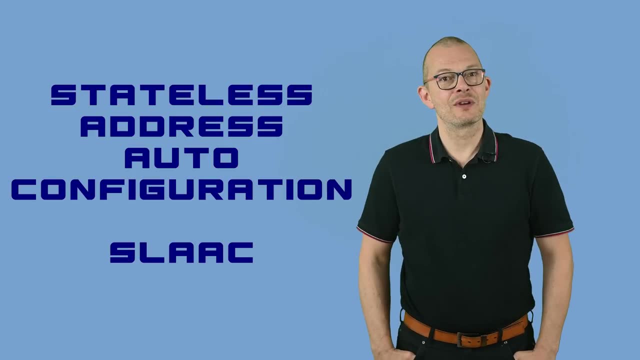 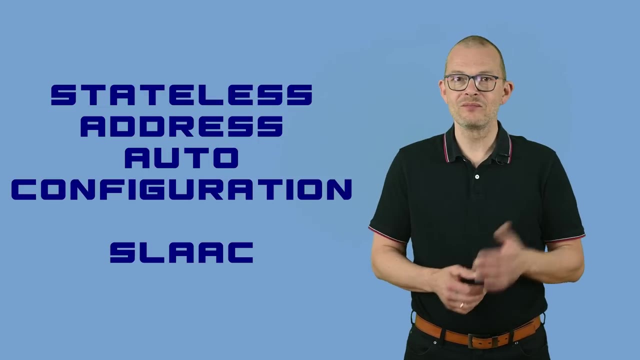 You know what? Let's actually allow them to generate IPv6 addresses for themselves independently, and we call that mechanism stateless address, auto configuration or slack. The IPv6 address is stateless because it comes from nowhere. We would just need to make sure that they are unique. 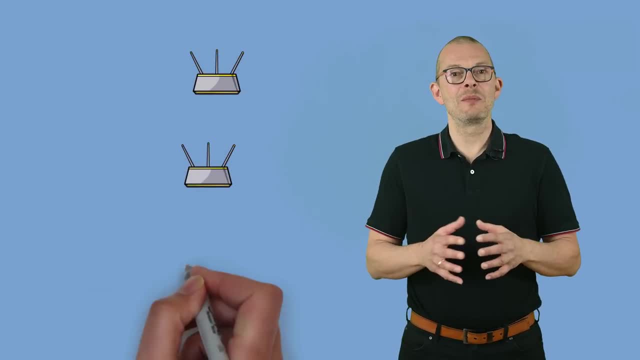 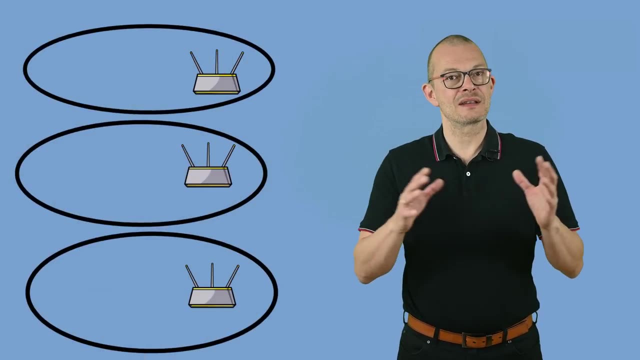 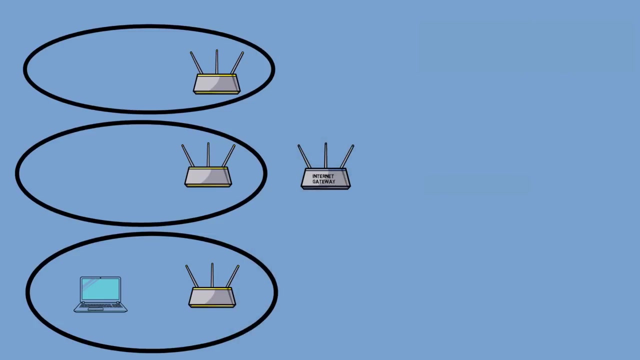 Actually, let's make our IPv6 network a bit larger in order to see what we need. Let's say we had a bunch of IPv6 routers here. They form IPv6 subnets. That means that they divide the network into smaller IPv6 networks And actually we could define three, or actually four different ranges or areas. 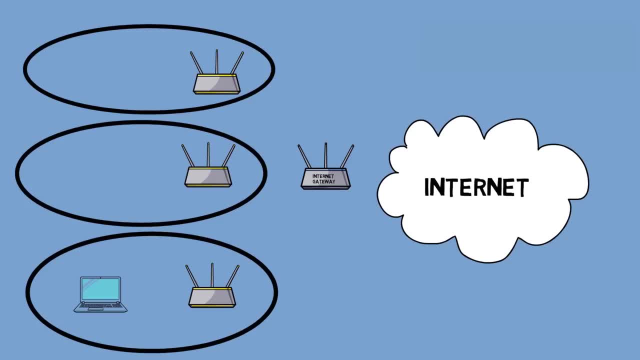 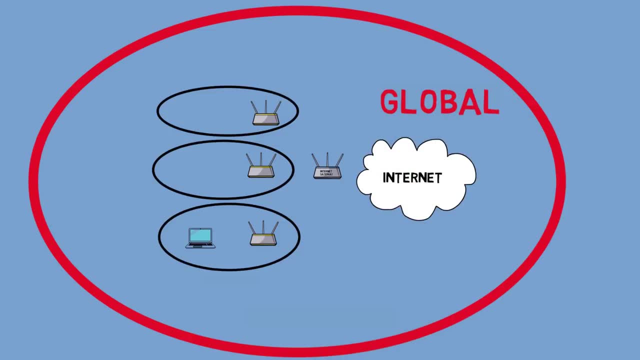 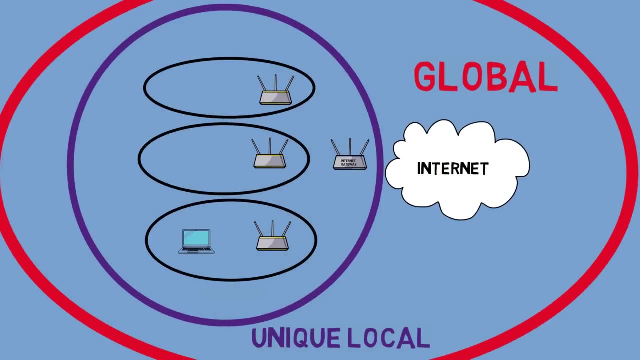 or let's call them IPv6 scope. One would be the internet. Let's call this IPv6 scope global. Now, inside our network, behind the internet gateway, we could basically do whatever we want. Let's call this IPv6 scope unique, local And if all hosts are on the same collision domain. 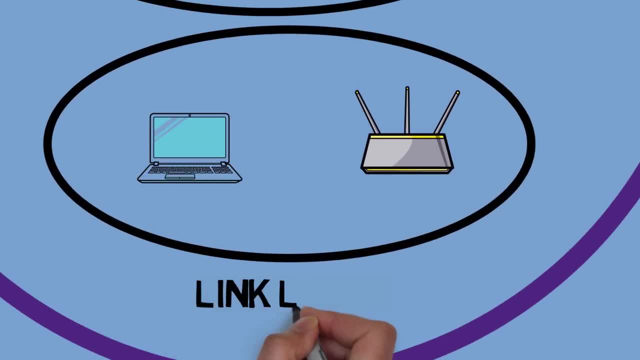 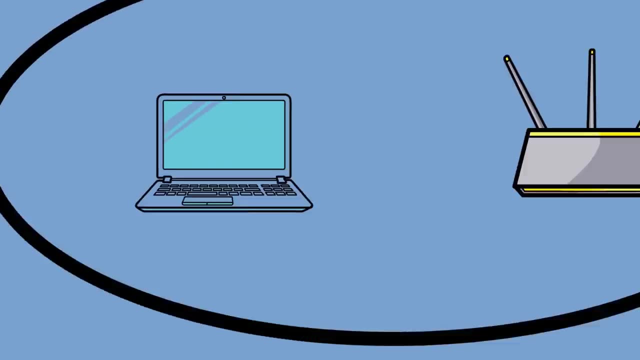 or in other words, in the same subnet or on the same switch, they share the same local link. Let's therefore call that IPv6 scope link local. If we go further to the inside, then we might add a fourth IPv6 scope and call that one local host. 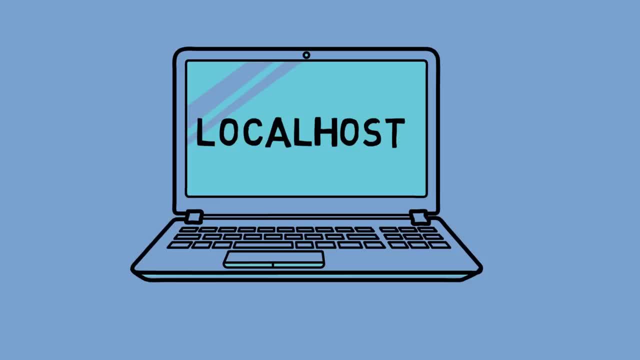 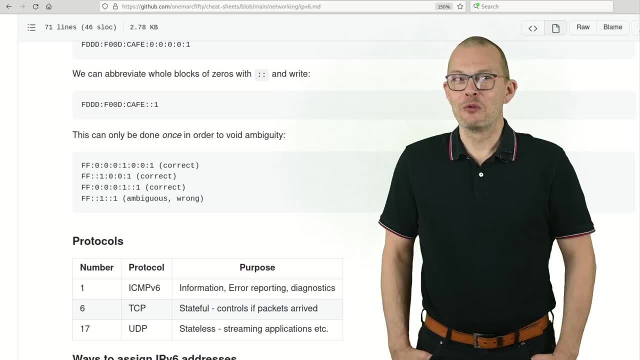 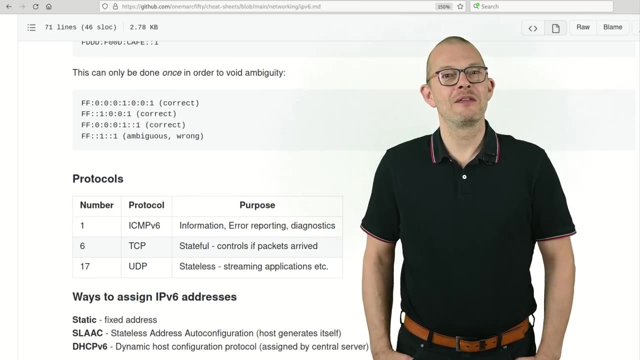 That would be the machine itself, For example, a user connecting with a web browser to a software that is running on the very same machine. Awesome, We are making great progress with our IPv6 protocol. I am positive that at the end of this video we have the perfect IPv6 protocol. 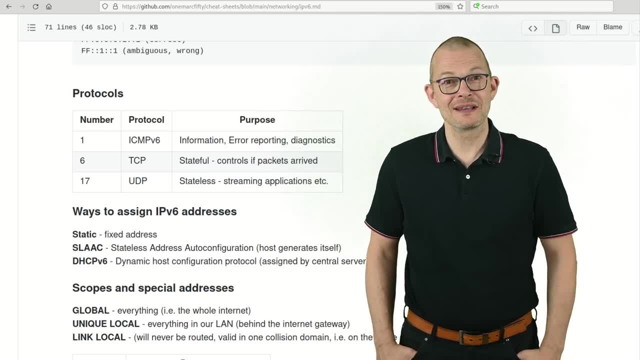 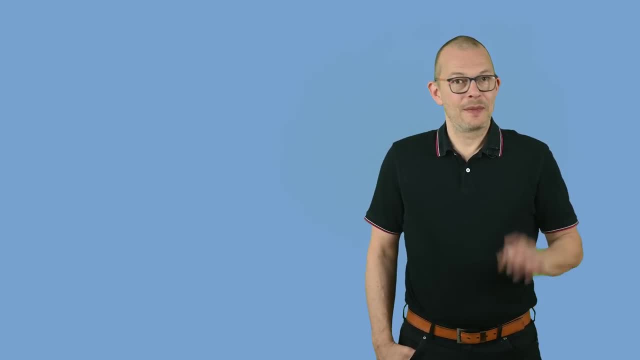 stack, Quickly writing everything into the IPv6 cheat sheet. Here we go: Scope and meaning. Now we thought that we had one challenge, but actually that leads us to a couple more things. First, how would the machine know which scope it is in? Let's actually solve this by defining address ranges or blocks. This 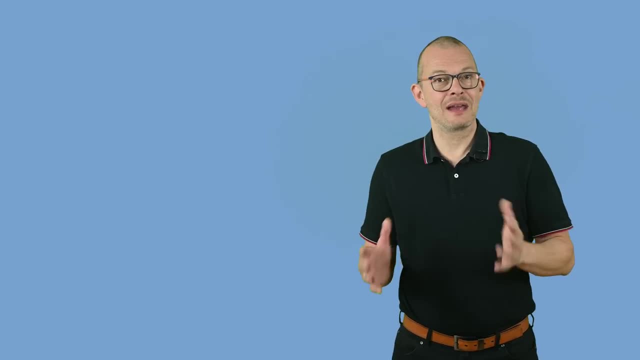 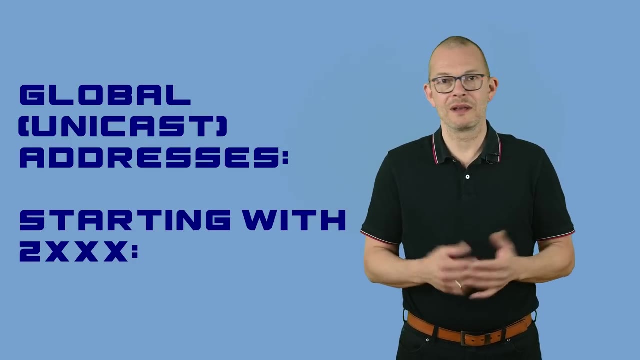 way a node would know the scope just by looking at the address. We arbitrarily choose the following address blocks: Let's start with, say 2001 and then go on – 2002 and so on. Let's assign blocks inside to different ISPs or Internet Service Providers If we need additional IPv6 blocks for special. 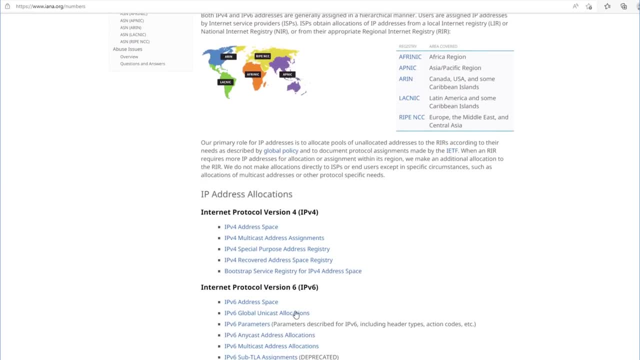 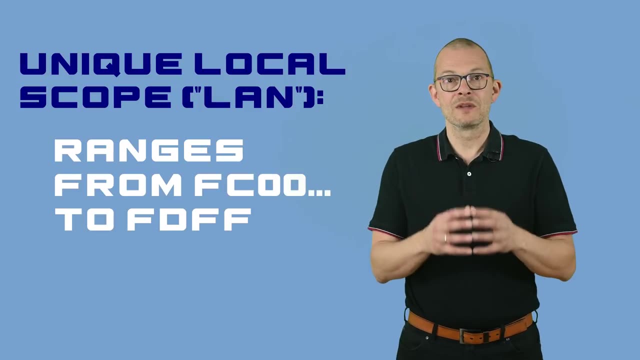 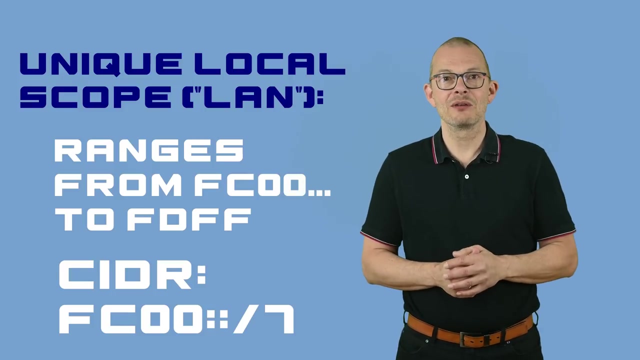 purposes, then the Internet Assigned Number Authority – the IANA – shall manage that. The unique local IPv6 scope shall get the range fc something to fd something or in classless internet domain routing, CIDR annotation: fc double zero. colon. colon slash seven because the first seven 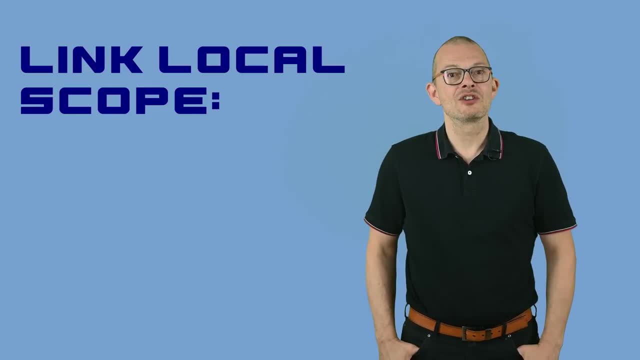 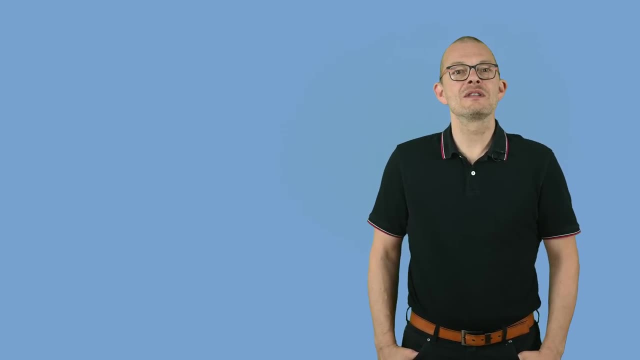 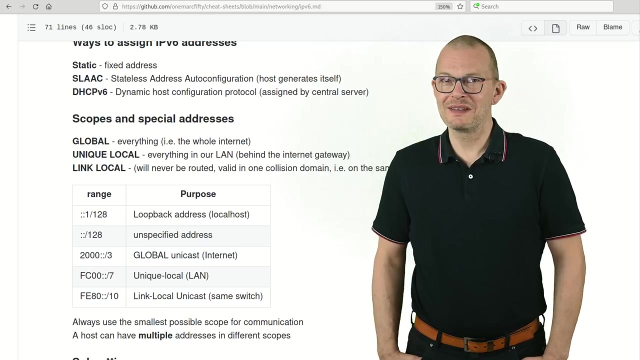 bits are significant here. The link local scope shall get the fe80 colon something range For the local host. let's use the most simple thinkable address – colon, colon one. Before I forget it, we want to write this into our IPv6 cheat sheet – address blocks. Here we go. 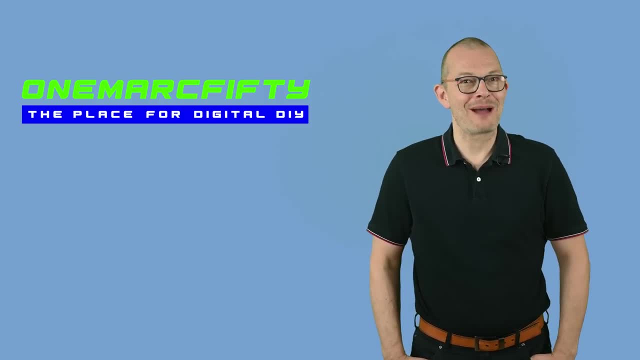 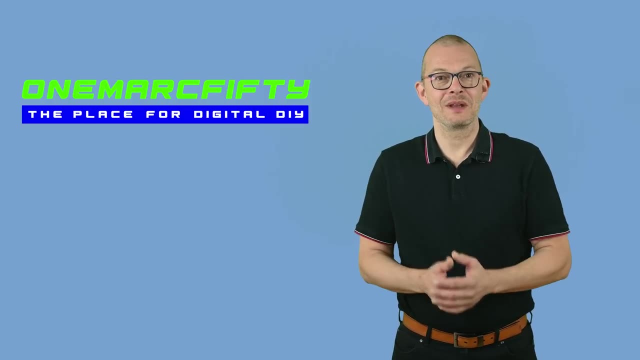 So now we can do the first thing. We can bootstrap or kick off IPv6 communication with address that the IPv6 node creates for itself – inside the link local scope – the fe80 range. To make sure that the IPv6 address is unique, the node can use, for example, its MAC address or a UID or 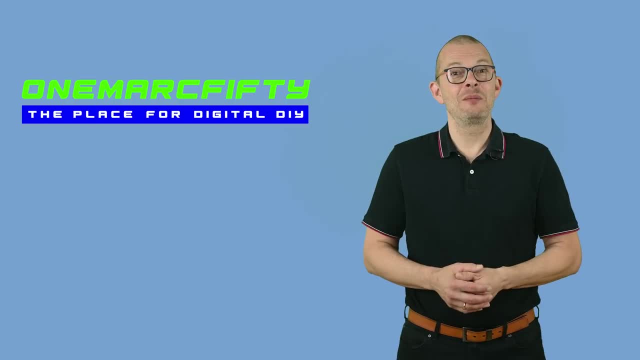 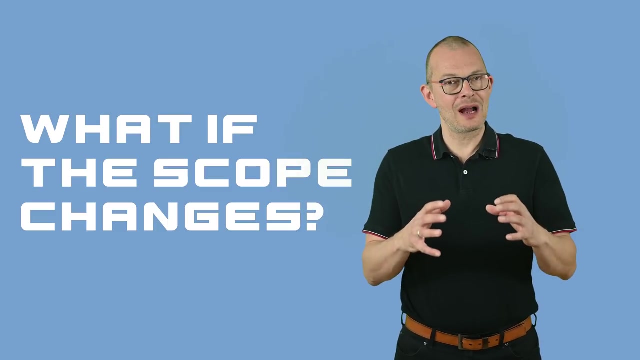 a timestamp or similar. From now on the IPv6 node can speak to the first IPv6 router, which in turn could then give out another IPv6 address in other IPv6 scopes. But then, if a router goes down, would we then need to change the IPv6 address from the global range to, let's say, link, local range? 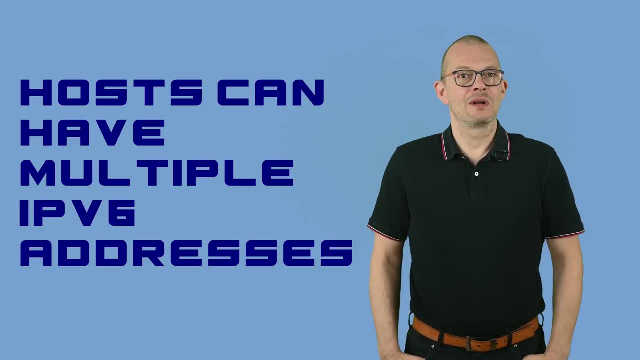 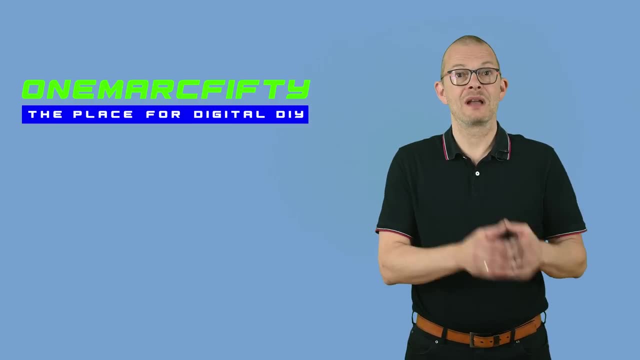 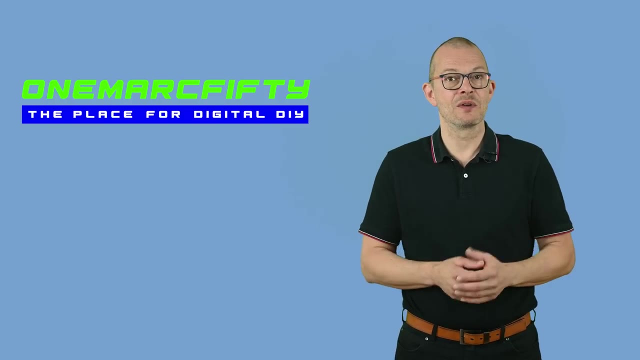 You know what? Let's solve this in another way. Let's allow nodes to have multiple IPv6 addresses, So a node will always have the local host address and a link local address starting with fe80.. Potentially, a unique local IPv6 address starting with fc or fd. Plus it could have a public or 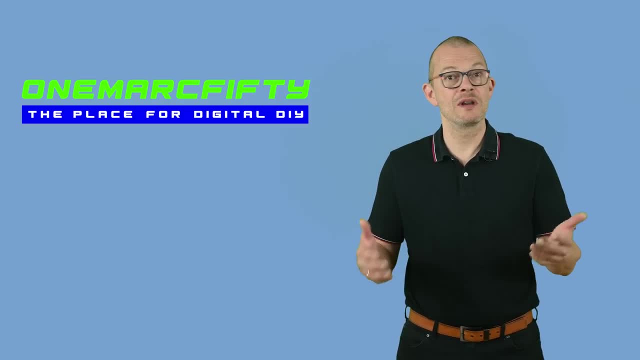 rather global scope IPv6 address starting with fe80.. So let's solve this in another way. Let's say we have 2 or 3 or maybe 4 at some point in time. In other words, if you see multiple IPv6 addresses on your host, if you type in ip addr or ip config slash, all in windows – don't panic. 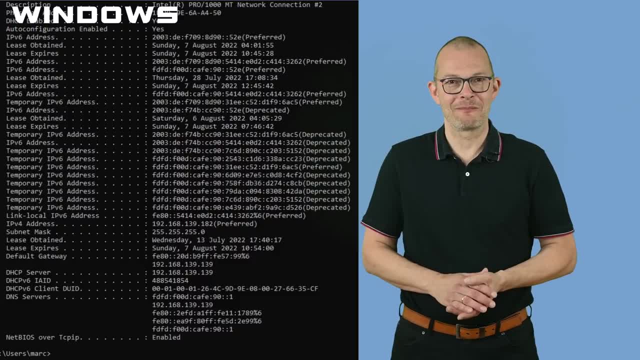 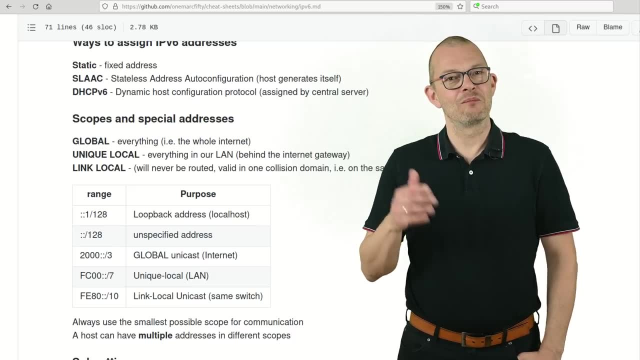 that's by design. Here is what that looks like on my PC. Let's quickly write all this down in the cheat sheet: Address ranges per scope, multiple addresses Plus. let's make a definition here in order to optimize traffic. Let's say: if two: 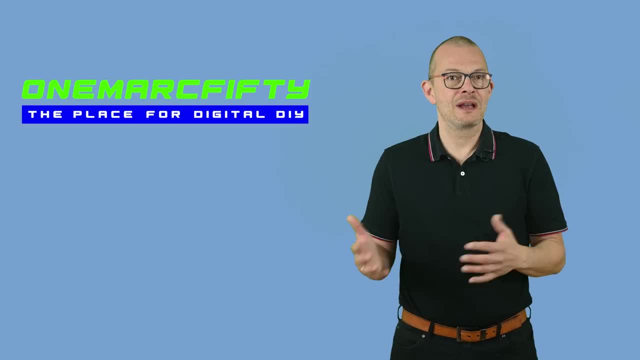 nodes are in the same subnet, then they should use the fe80 IPv6 address to communicate. That will avoid that routers need to route local traffic that could have gone over the switch. So I add to the IPv6 cheat sheet: – always use the smallest possible scope for communications. 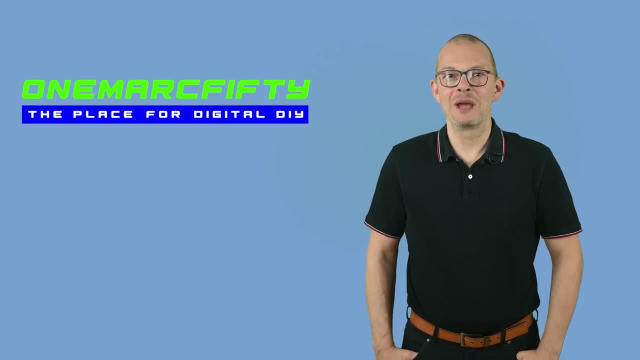 What is missing to make the perfect protocol. Maybe we should add a couple of mechanisms for subnetting here. As we have so many addresses, we can be utterly generous in giving them away. Let's say we cut the IPv6 address in half. The first half of the IPv6 address would identify the network and the second half the node. So all nodes in one network would share the same four identical first blocks and could have four unique blocks for the IPv6 address inside the network or for their interface. I should say, Actually, let's even go. 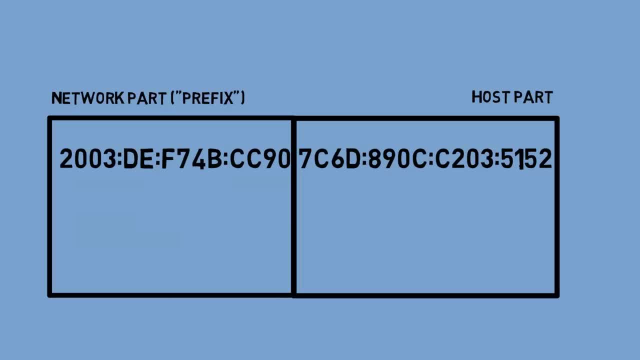 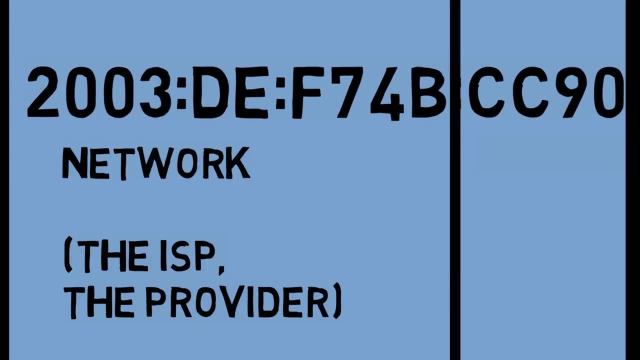 further. We don't have that many networks or providers. I should say in the internet 6 bytes or 48 bits will be enough to determine the site or the ISP or the backbone where a packet needs to go in the internet. That will drastically speed up routing in the internet. We can then use 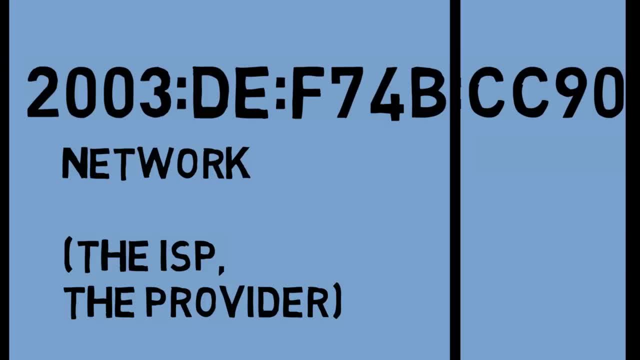 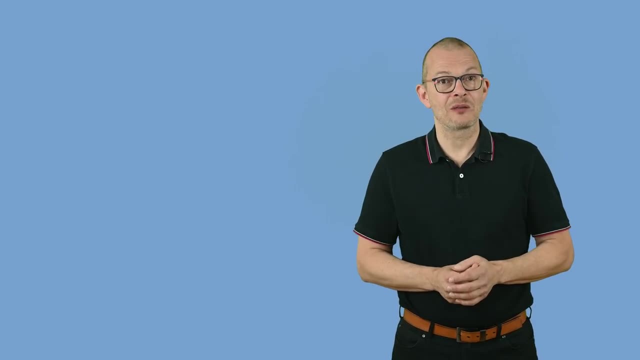 the remaining 16 bits of the first block for networks, or rather subnets. We could even give whole IPv6 networks to the subscriber – the consumer – you know the user Here in Germany, Deutsche Telekom, who have the 2003 something network. 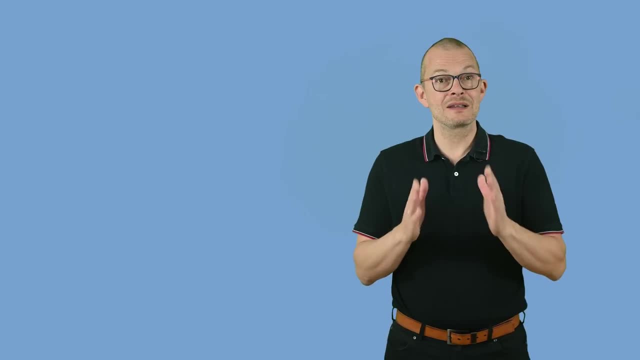 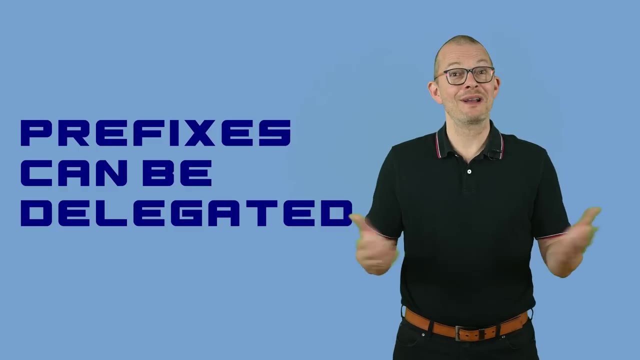 actually allow me, as a simple consumer, to use the last 8 bits for subnetting. That means they are delegating a 56 bit prefix to me which I can use for subnets as I please. I can therefore create 256 subnets with zillions of public IPv6 addresses inside. Amazing how big the thing is. 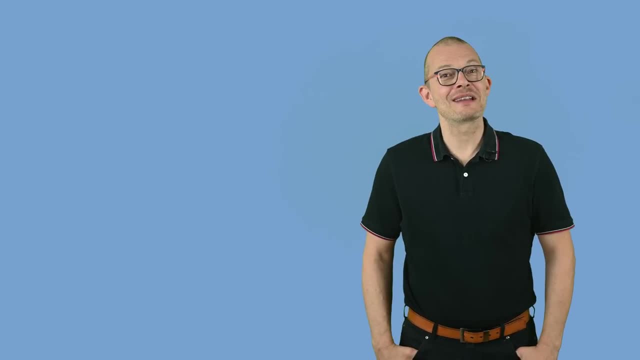 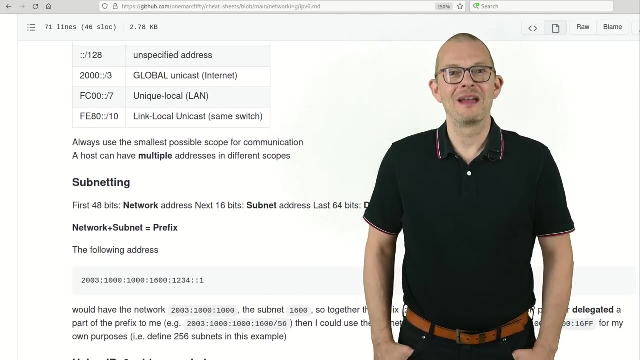 6 bits of the IPv6 address will be enough to determine the site or the IPv6 address inside. Cool, Let's stop here and summarize our findings on the cheat sheet: Subnets, Prefixes, Interface addresses. Before we close, I quickly want to show you a couple of very basic IPv6 tools. 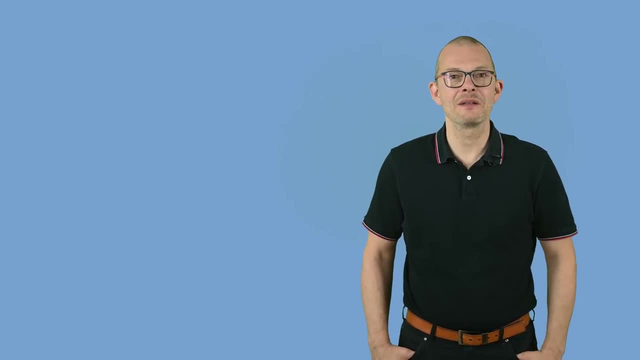 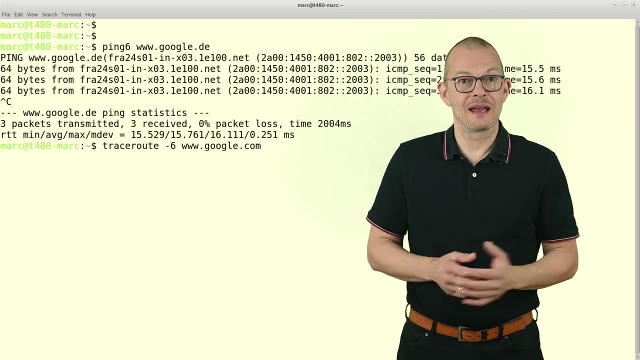 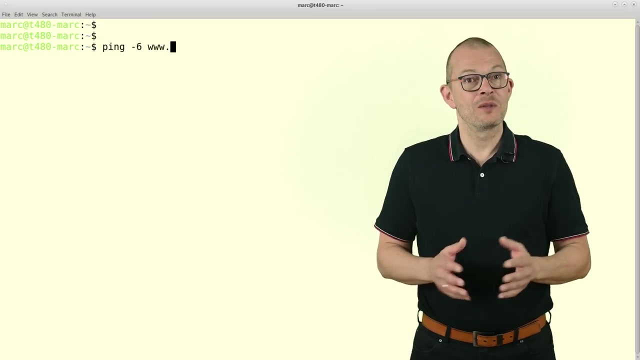 that you of course know already. They are the same like in IPv4 – you may now remember it again, Just on Linux, they very often have a 6 at the end in order to indicate IPv6 usage, such as ping6, or traceroute6.. Or, with many of those, you can just add –6 in order to tell the tool to use. 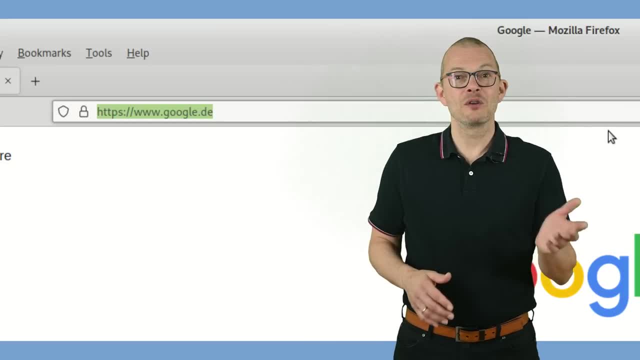 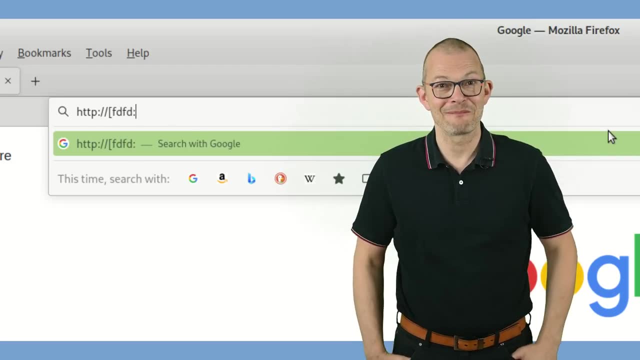 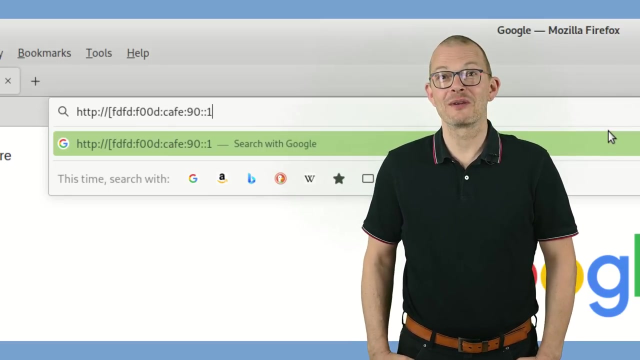 IPv6 rather than IPv4.. If you want to open a web page's IPv6 address, then you can just write the address into the browser's address bar with square brackets. Guys, that's it for today. We have successfully designed the IPv6 protocol from scratch. I hope you liked the episode. If so, 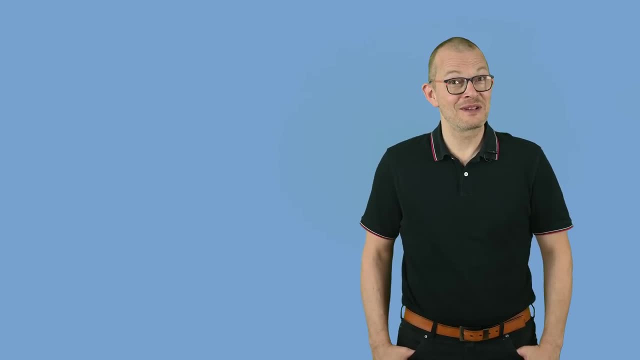 a like on YouTube is much appreciated. Thanks for watching and see you next time. Bye, bye. In one of the next episodes I will show you how to configure IPv6 with OpenWrt Plus. we might want to see how we can transform our IPv4 ARP spoof device into an IPv6 network analyzer. 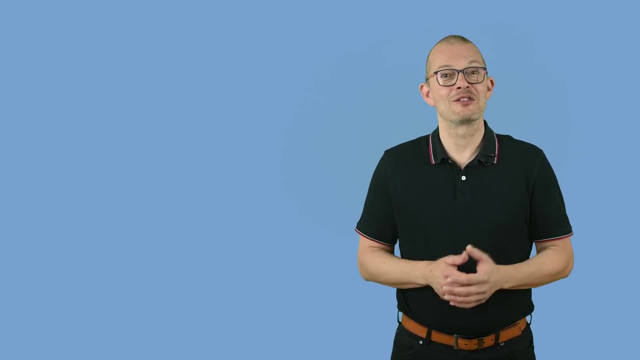 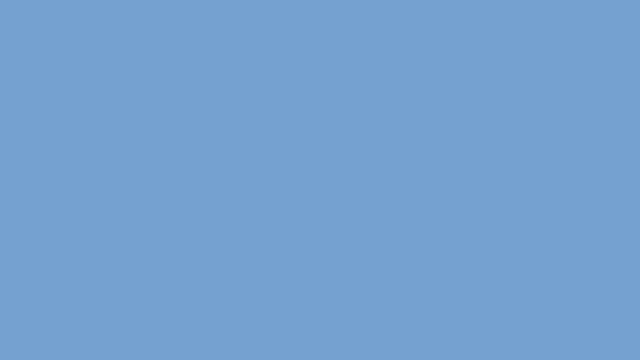 The link to the IPv6 cheat sheet is in the description. Many thanks for watching. Stay safe, stay healthy. bye for now. http//wwwyoutubecomsummitcomsummitcom. http//wwwyoutubecomsummitcomsummitcomsummitcom.